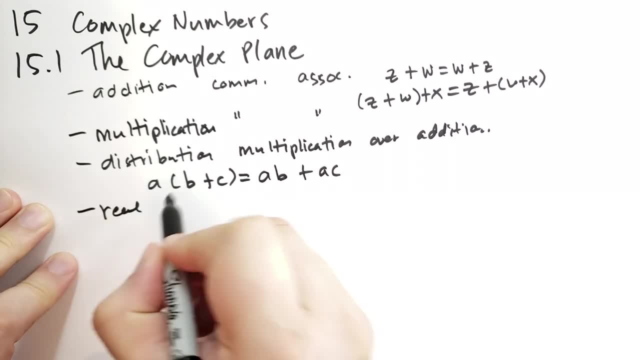 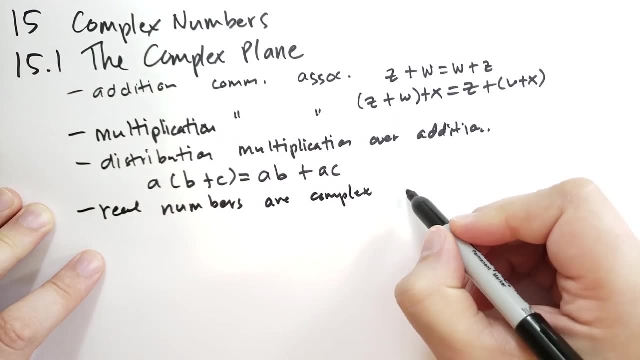 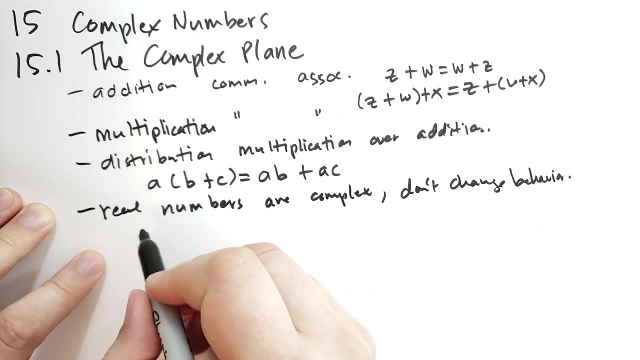 Okay. We also have the rule that the real numbers are part of the set And they don't change their behavior. That means that if you know a and b are real and you add a and b, you're going to get the same result as you always have. 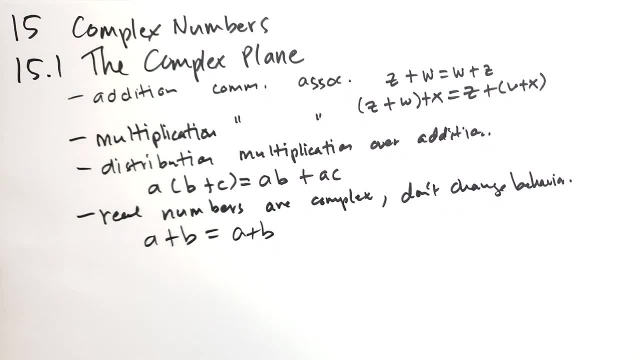 even if you consider it as a complex number. So nothing changes there. thankfully We also have one is a real number And it satisfies the property that one times any complex number- z is in fact that complex number We also have. zero is a real number. 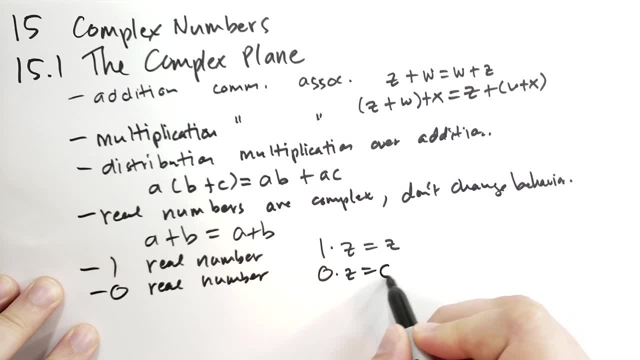 And a complex number. We have zero times z is going to give you zero, And zero plus z is going to give you z back as well. It's the identity for addition. There is also an additive inverse, So we have negative z plus z is equal to zero. 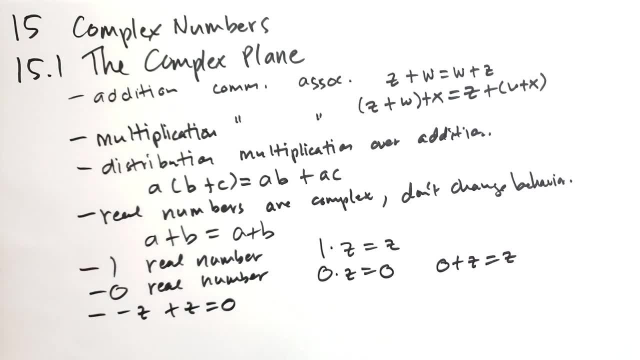 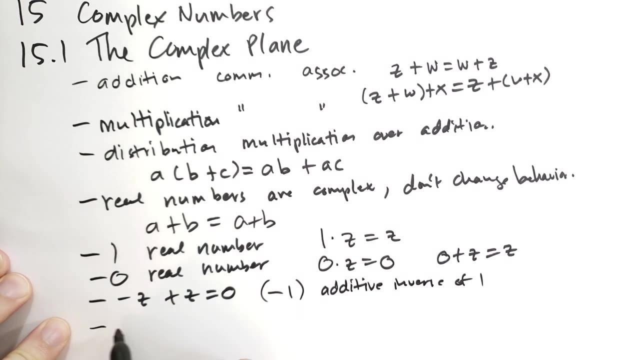 So we can add numbers that will cancel the other number out. So negative one is the additive inverse of one. There exists a complex, There is a complex number i, such that i squared is equal to minus one. i squared is equal to minus one. 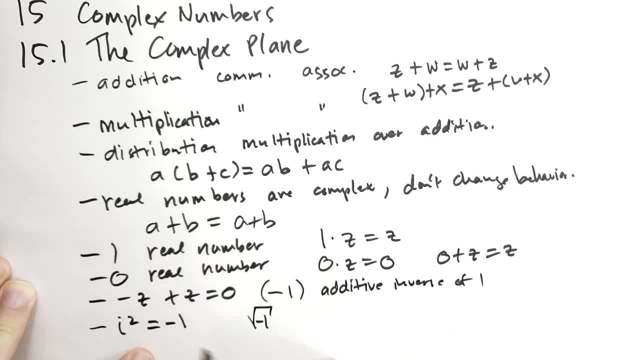 Note, however, that the square root of minus one under this system is equal to. It can be i or negative i. If you take negative i and square it, you'll also get negative one. This confuses a lot of people, And there's actually people out there on the internet saying that the complex numbers don't work because of this little thing here. 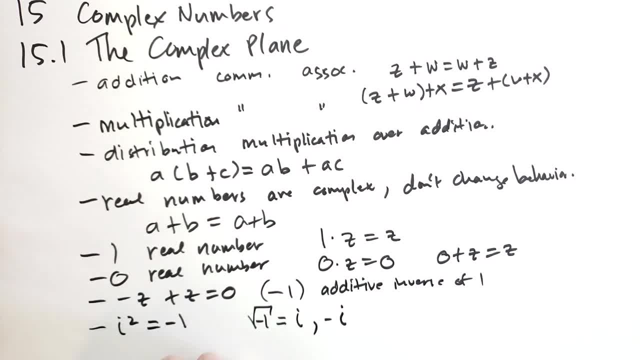 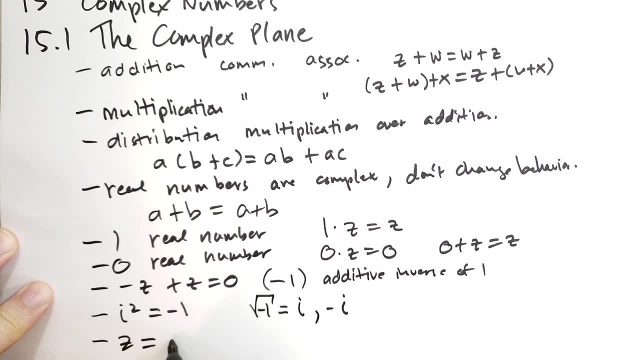 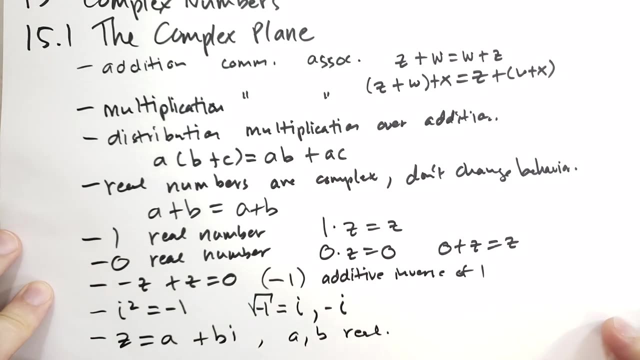 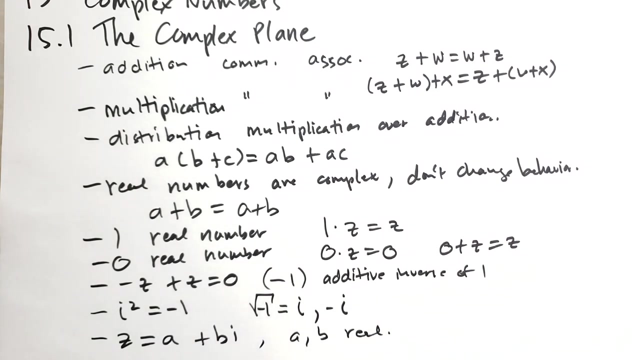 Okay, And finally we have the last And most important rule in the complex plane is that every complex number, z, can be written as a plus bi, where a and b are real. Okay, If you're not familiar with the terminology here, real numbers are all the integers, all the rationals, which are integers divided by integers. 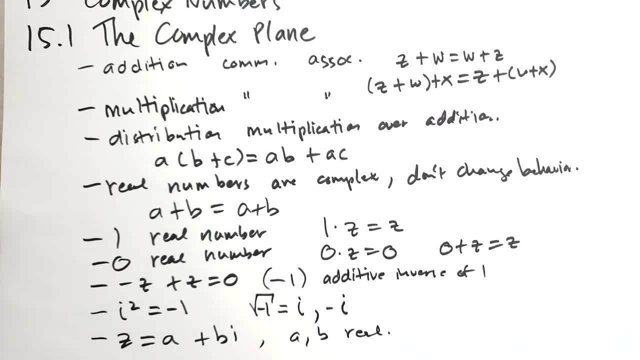 and all the irrationals, like square root of two and pi, those numbers that can't be expressed as ratios of integers. So the real numbers are now. So the real numbers are now. So the real numbers are now going to be supplemented. 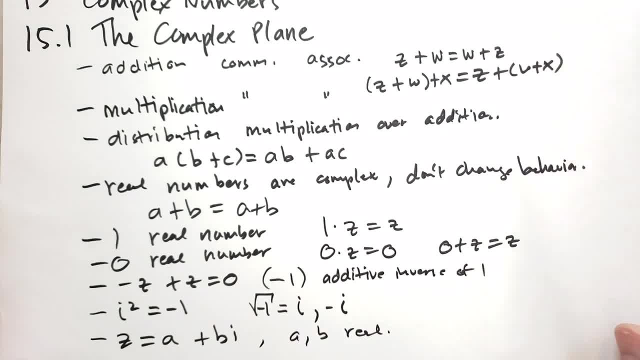 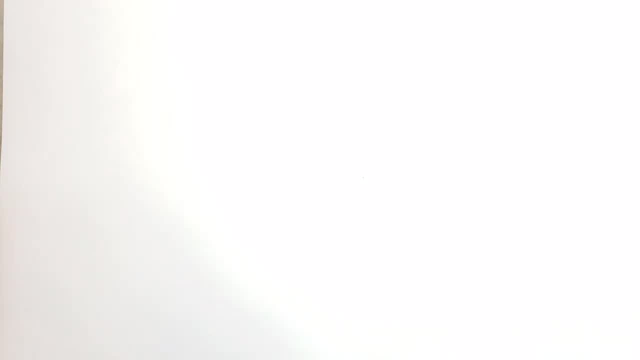 We have complex numbers that have all of these curious behaviors, So let's get to it and see what happens because of these things. Okay, All right, We have. Just as we represent a real number as a line, we can represent complex numbers in the plane. 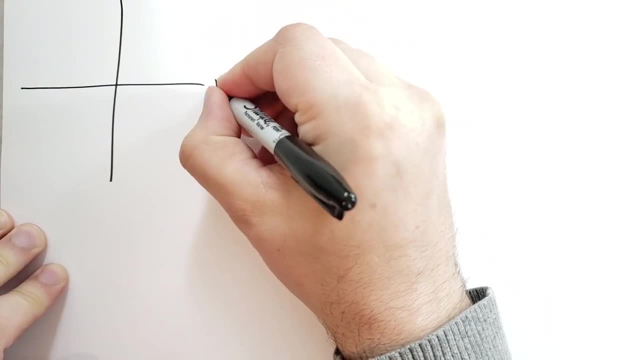 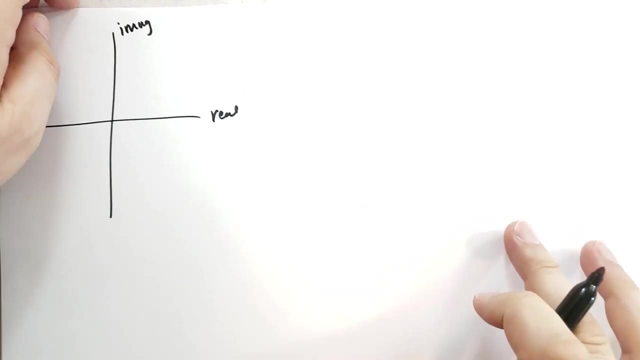 So let's draw a plane here, And what we're going to do is we're going to call this the real and we're going to call this the imaginary. Okay, Let me scroll that down there so you can see. Okay. 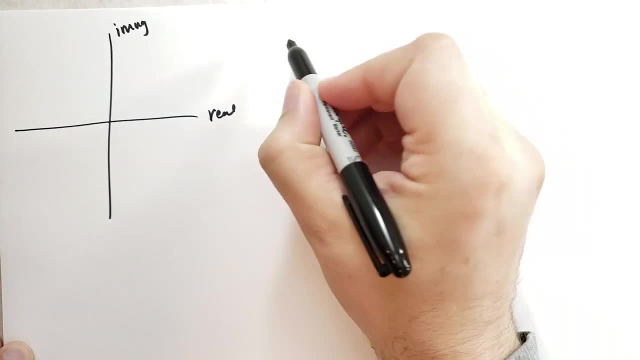 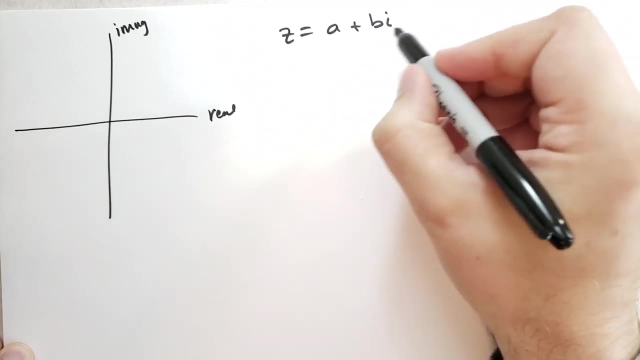 So let's suppose that we had any number z equals a Plus b, i, In which case in the complex plane this number would be represented by the coordinates a, comma, b. Note that a and b are real numbers. 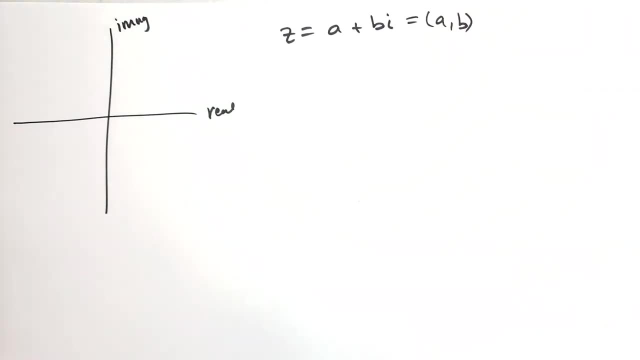 They're not imaginary or complex or anything like that. As an example, let's say we had z is equal to 3 plus 2i, So we go 1, 2, 3 over and 1, 2 up, and that would be z. 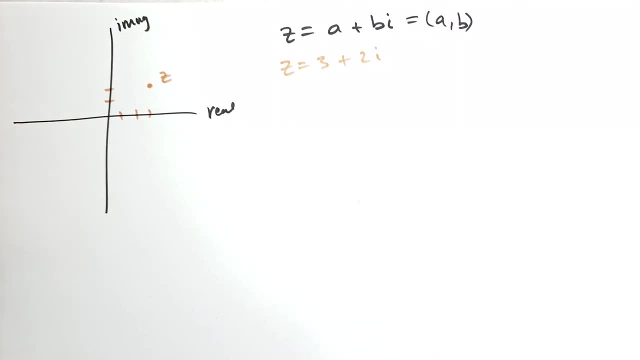 Okay, Okay, Okay, So we have i represented by 0, comma 1.. So this is i right there, Okay, 1, obviously is represented here. Okay, Hopefully this isn't terribly confusing. You can play games and figure out where all the different numbers end up on this complex plane. 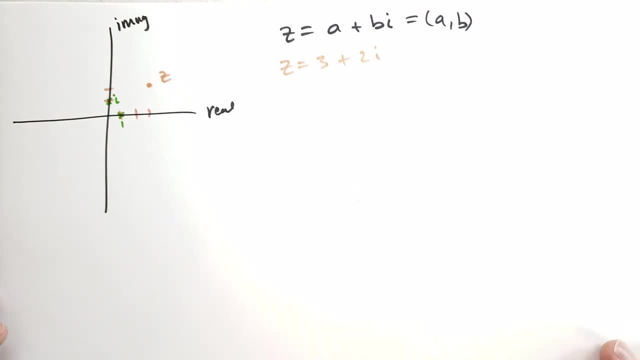 It is important to note that you can no longer represent complex numbers as a line, And so it's kind of pointless to ask which complex number is bigger than another. It doesn't really make sense in this context anymore. Okay, If we had 2.. 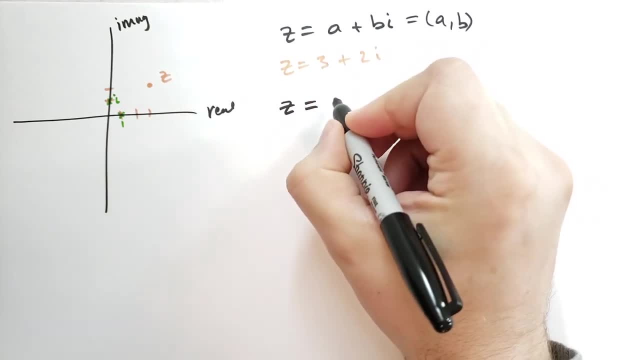 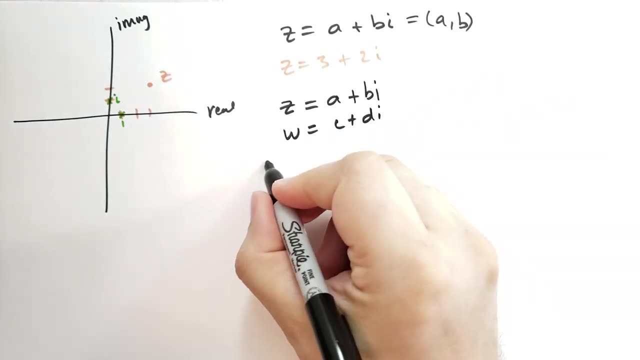 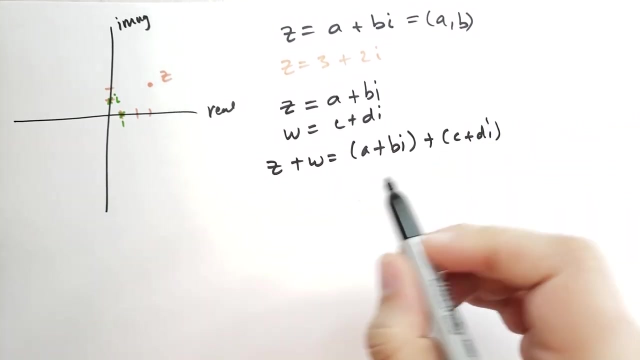 Numbers z, which is equal to a plus bi, and w, which is c plus di, And we wanted to add these two numbers together. Let's take a look at what would happen. Okay, So we write it out this way. 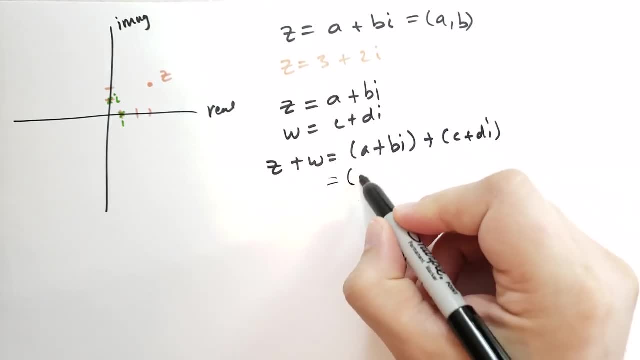 We note that there are two real terms. So we have a plus c And we have bi and di. that we add together, So we get b plus di. So the net effect is, if you think of these as points, let's say c, comma, d, 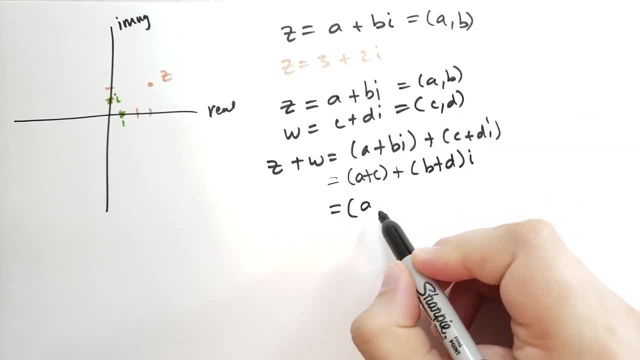 then adding these points is the same as taking the x-coordinate of the points or the real coordinate, and adding the complex or y-coordinate together Works just the way that you've learned when you add points together earlier in this book We also have, if we have a real number, c, and we multiply z by c. 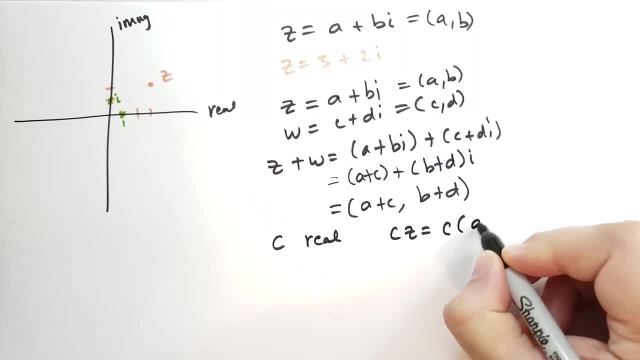 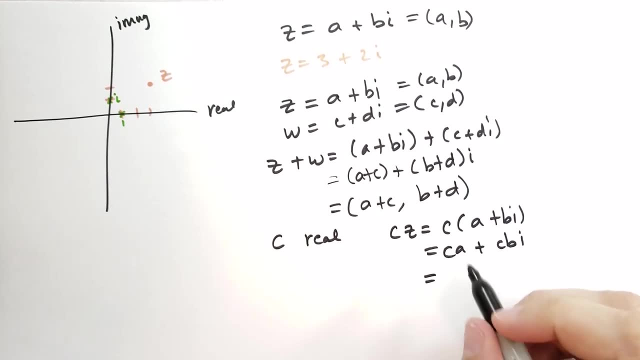 So we take c times z. What's that going to do? Well, you're going to have c times a plus bi And that's going to give you ca plus cbi. Or, if you think about this in terms of a point in the complex plane, that's just going to be ca, comma, cb. 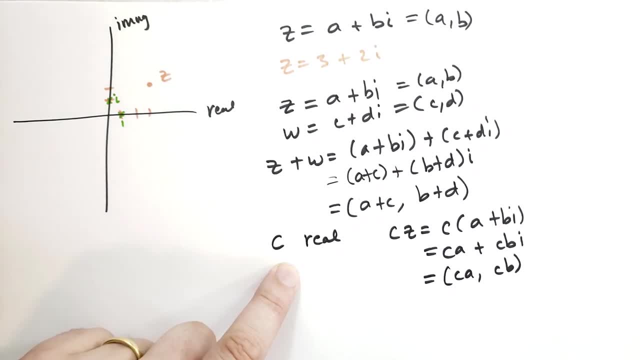 Okay, So that's scaling the point out by a factor of c, when c is real, If we multiply two numbers together. So let's say we have z times w. What's going on here? We have a plus bi times c plus di. 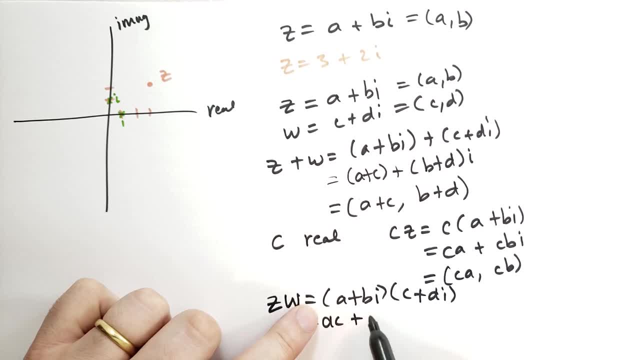 So we distribute these terms. We have a times c, We have b times c, So I'm going to call that bci. We have a times di plus adi And then bi times di, So bdi squared. 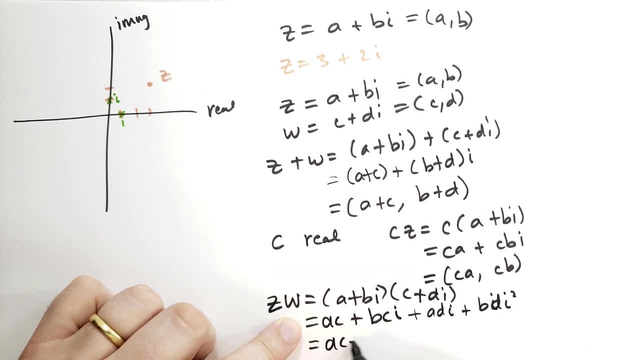 What's i squared? That's just minus 1.. So we have ac minus bd plus bc plus a. These are i's bd and adi, So we can rewrite this: ac minus bd plus bc plus adi. Okay. 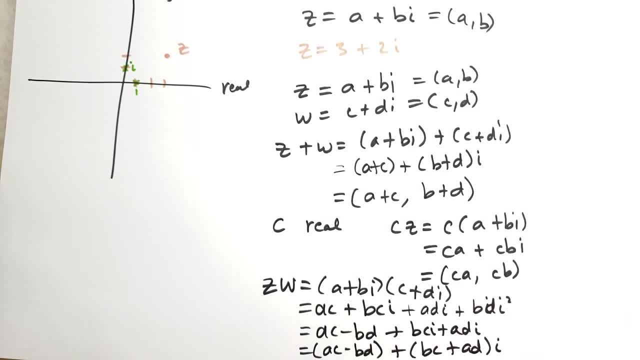 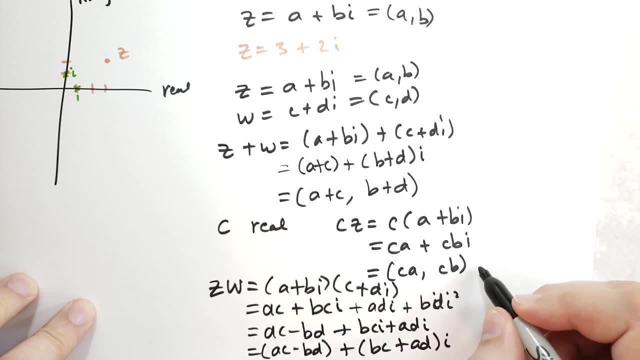 That's how you multiply two complex numbers together algebraically. Rule of thumb here is if you had these as a point, So let's draw this as a point. It's basically going to be a comma b times c comma d, Multiplying two points in the plane. 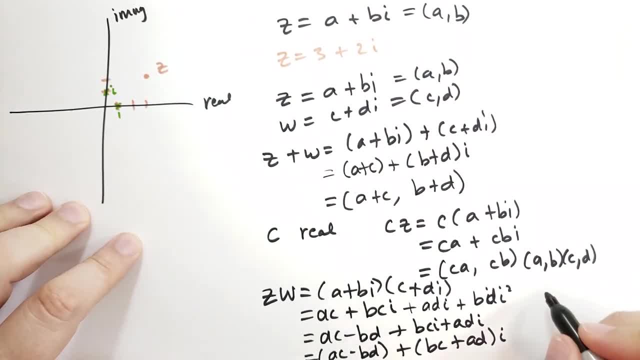 We haven't talked about that, what that means yet, And that's going to give you ac. let's make sure I get this right: ac minus bd plus bc minus bd, comma, bc plus adi. Okay, So it's going to be the real terms minus the coefficients of the complex terms. 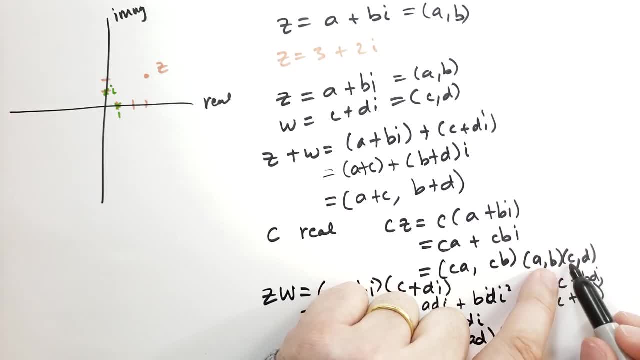 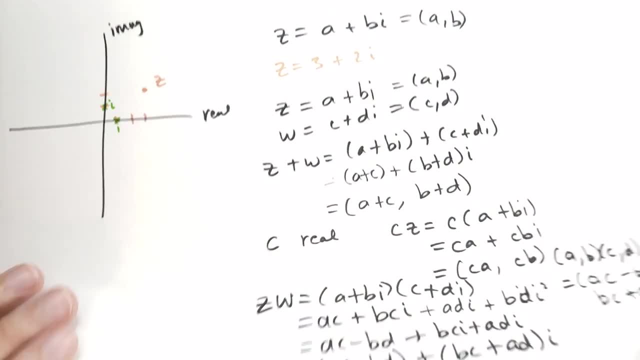 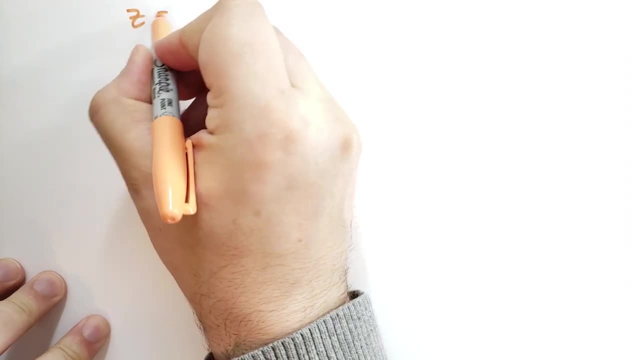 So the real components of the complex terms or the imaginary terms, And then you're going to take these two inside and outside terms and multiply them together for the imaginary part. As an example, let's do some complex multiplication. So we're going to take: z is equal to 2 plus 3i. 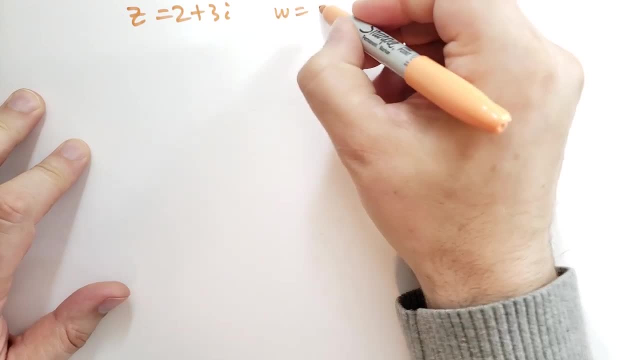 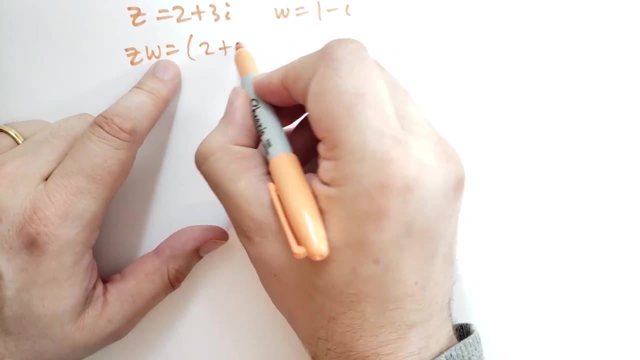 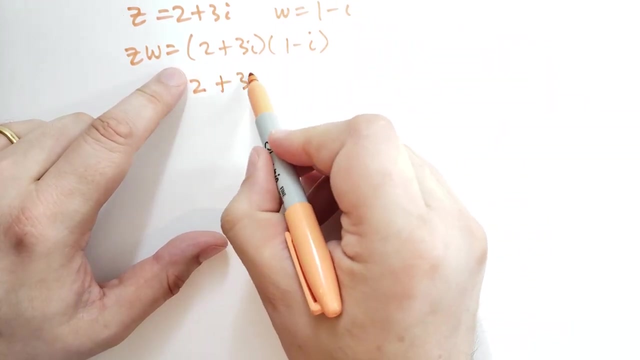 Can you all see that? Good, And we have w is equal to 1 minus i. The product of z and w together is going to be 2 plus 3i times 1 minus i, which is equal to 2 plus 3i. 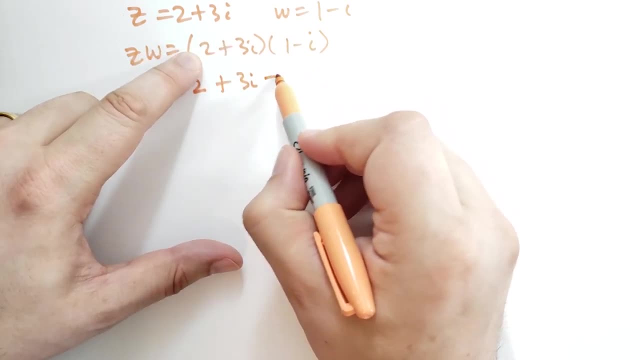 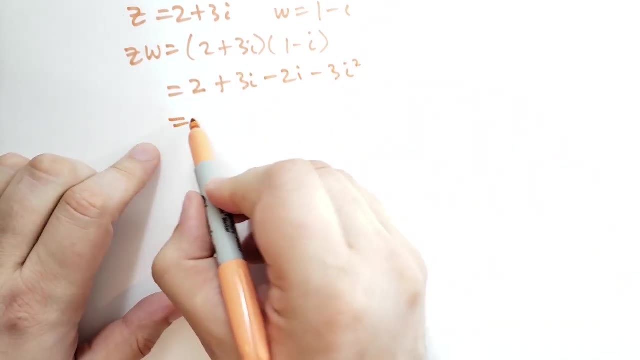 So these two terms, those two terms, and then we do these two terms minus 2i, and then this is going to be minus 3i Plus 3i squared, And since 3i squared is negative 1, this is going to be 2 plus 3 from this term, and we 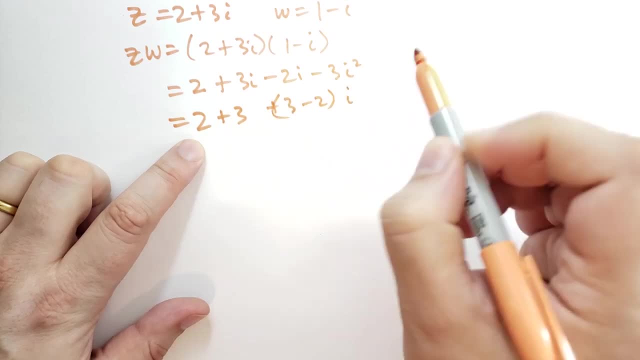 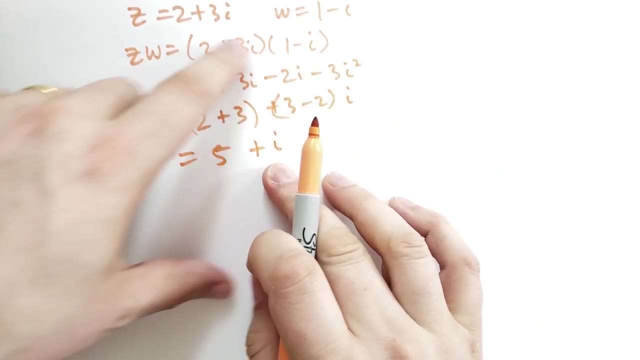 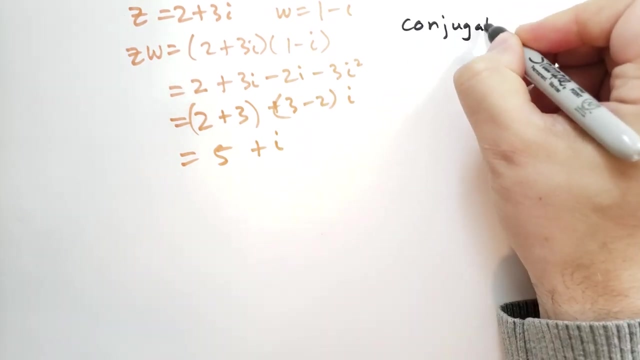 have plus 3 minus 2i. Okay, So this is going to be 5 plus i. That is the product of z and w multiplied together. Let's talk about the complex conjugate now. So the complex conjugate is written with a bar over the top. 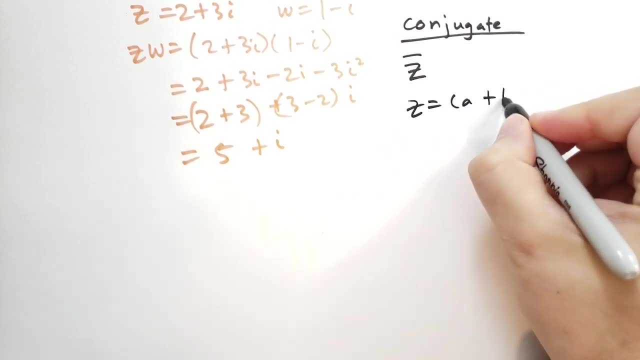 Okay, And if z is equal to a plus bi, then z with the complex conjugate is going to be a minus bi. Okay, That's what the complex conjugate does. Let's look at what happens when you multiply the complex conjugate together. 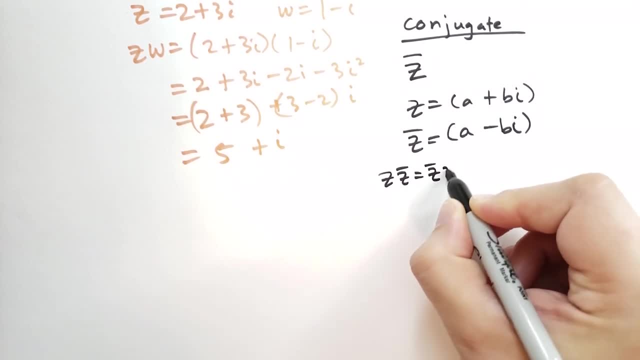 So we take z times z bar is going to be the same as z bar times z, which is going to be this term squared, and then we're going to have a times minus b and a times plus b added together, which is going to give you 0 for that. 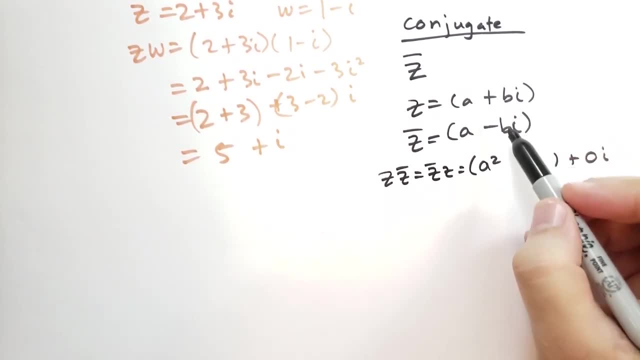 So there's no i component, And then, finally, we have these two terms multiplied with b times minus b squared, and then the i squared as well turns out to a positive. So the end result is this is going to be a squared plus b squared, which you might 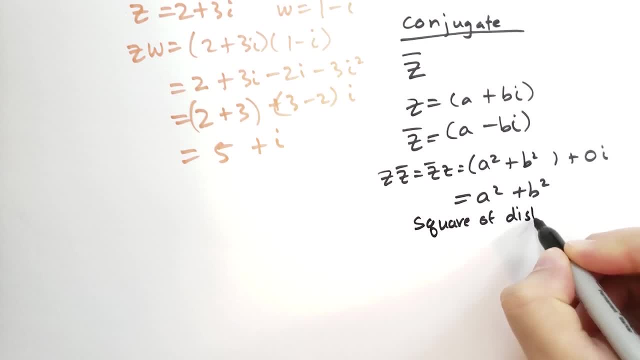 think of as the square of the distance from 0 comma 2.. Okay, 0 comma 0, which is the origin to z in the complex plane? Okay, That'll be useful later. What is the multiplicative inverse of z? 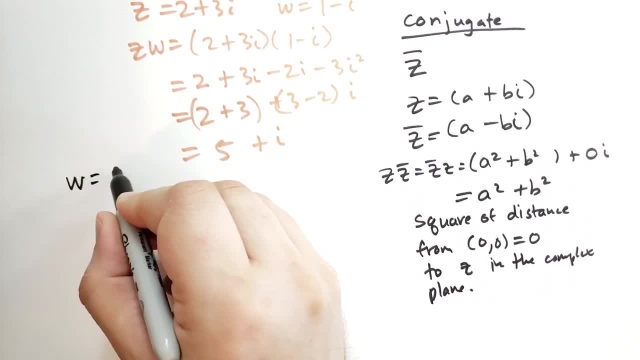 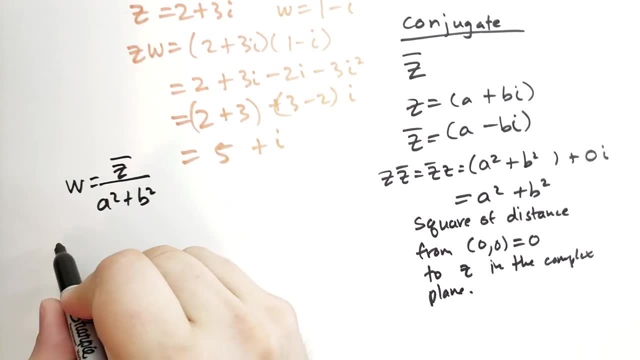 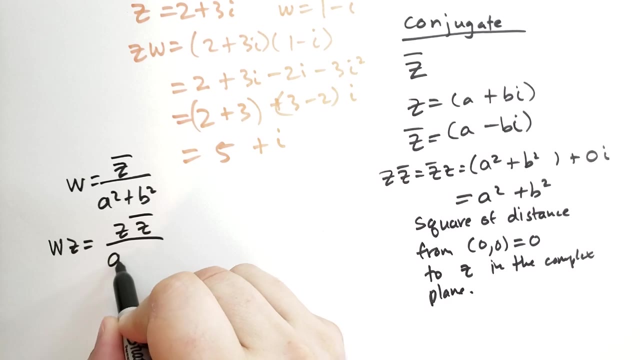 Okay, So let's suppose we had w which is equal to z bar divided by a squared plus b squared. Where did I get these numbers? Just bear with me, See what happens When we take w times z. We're going to get z times z bar over a squared plus b squared, which is going to be a squared. 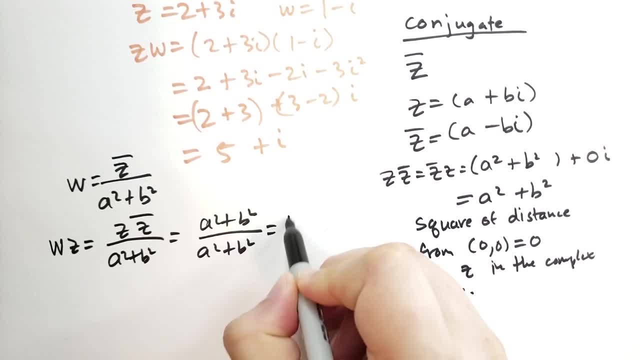 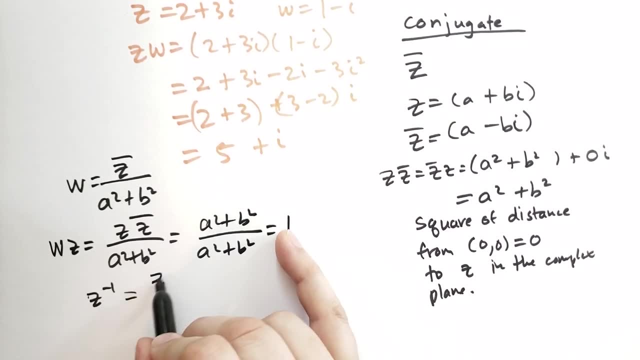 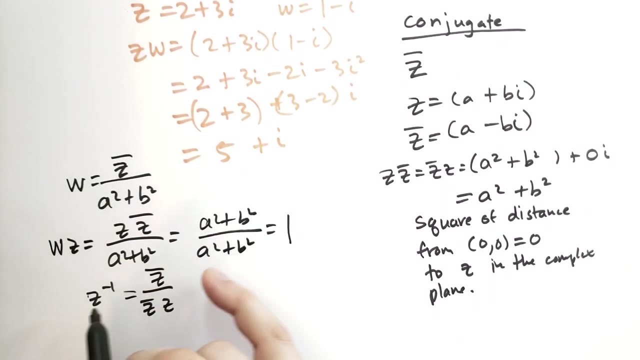 plus b squared over a squared plus b squared, which gives you 1.. So z, the multiplicative inverse of z, is the same as z bar over z z bar. Okay, Another way to think of this is the multiplicative inverse is 1 over z. 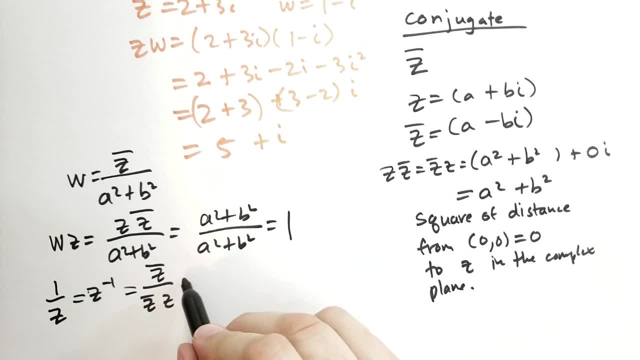 So that's what we do. So one more time: z bar over a squared plus b squared. Okay, That's how you find the multiplicative inverse And you can prove for yourself that there's only 1.. The way you do it is you say, if we had w times, z is equal to 1, and let's say there was another. 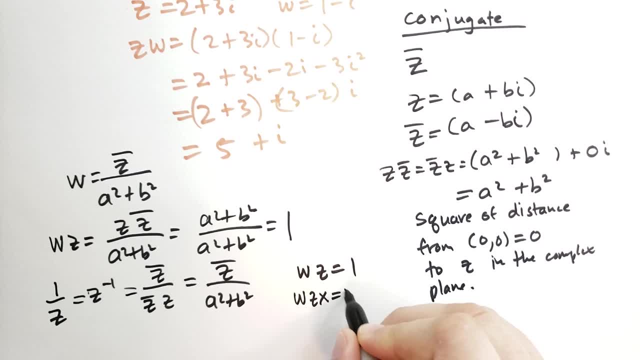 one wx. So we have w z times x should be equal to x. Well, that means that w and z times x. If x is the multiplicative inverse, If x is the multiplicative inverse of z, then that's just w equals x, because that's 1.. 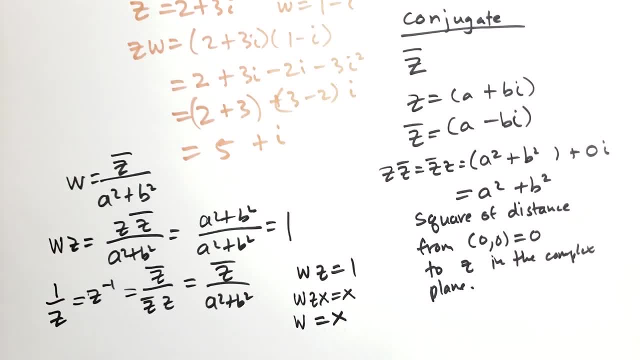 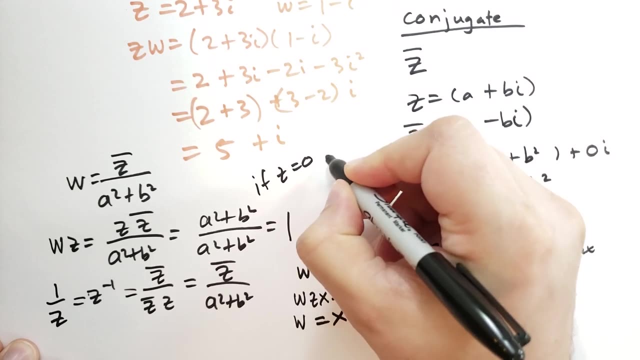 w times. 1 is w, and so you get w equals to x. So you prove that w is unique. There is no other complex number that you multiply a complex number by to get the multiplicative inverse. All right. Note that this doesn't work if z is equal to 0. 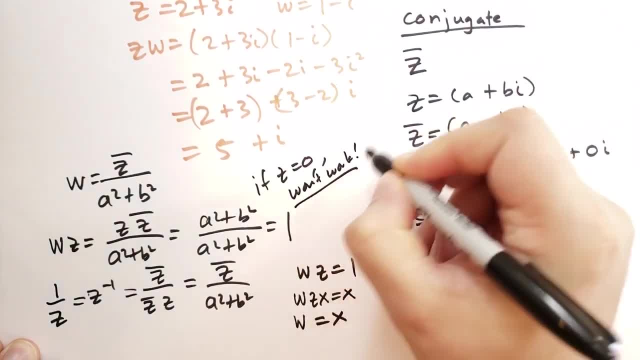 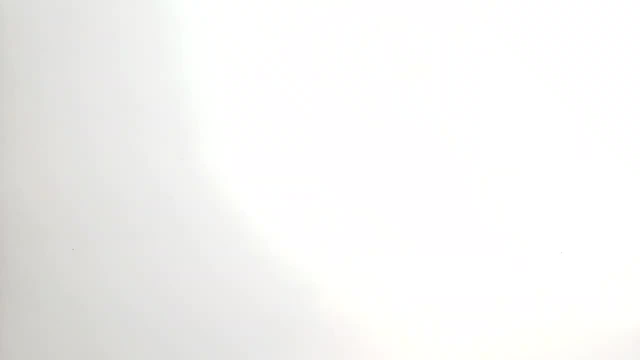 This won't work, Okay, Because a and b would be 0, and you'd be dividing by 0.. All right, So you can do that if z is equal to 0.. Let's do a little problem here as an example. 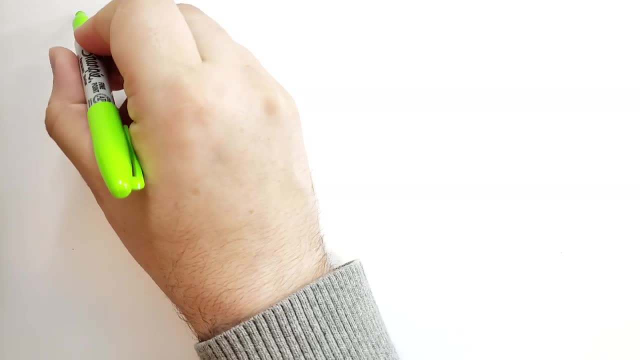 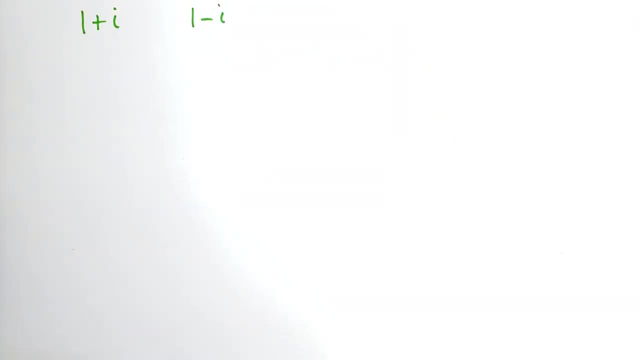 So we have the inverse of 1 plus i. What's the inverse of that, Right? So the conjugate is 1 minus i, and a squared plus b squared is 2.. Okay, So 1 plus i times 1 minus i, all over 2 should give you 1.. 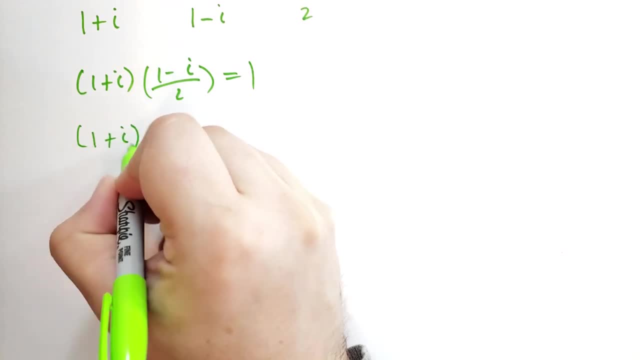 Okay, Another way to think of it. If we took 1 plus i and we multiply that times 1 minus i, what will we get? Well, we get 1, and the i terms would cancel, because you have plus i here and minus i there. 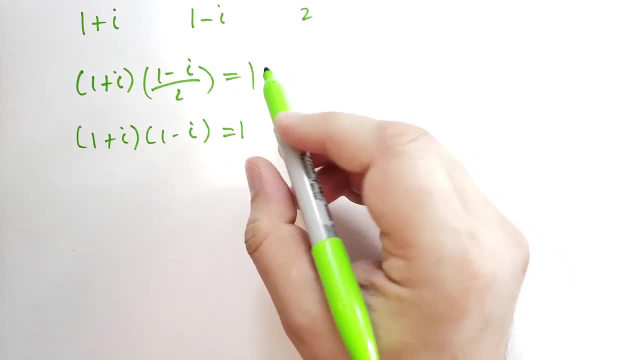 You'd have plus i times minus i. So minus i squared, which is 1.. Minus i squared is 1.. Yes, So we get 1 plus 1, which is equal to 2.. And so we want the multiplicative inverse of this. 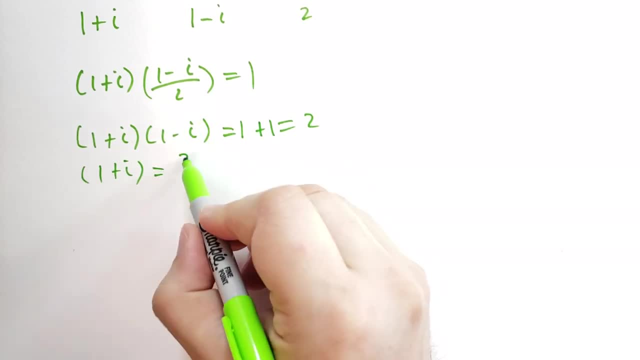 So we say 1 plus i is equal to 2 over 1 minus i. Or you can just reverse it and say the inverse of this: 1 minus i to the minus 1 is going to be 1 minus i, all over 2.. 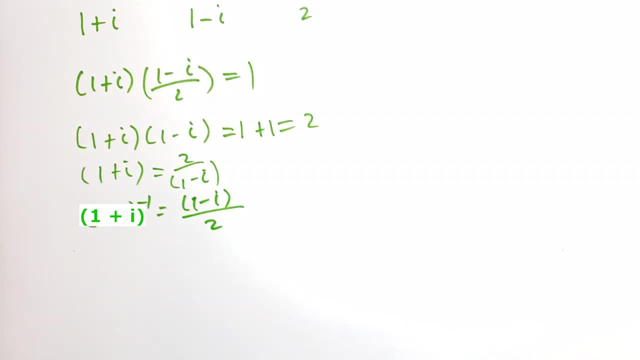 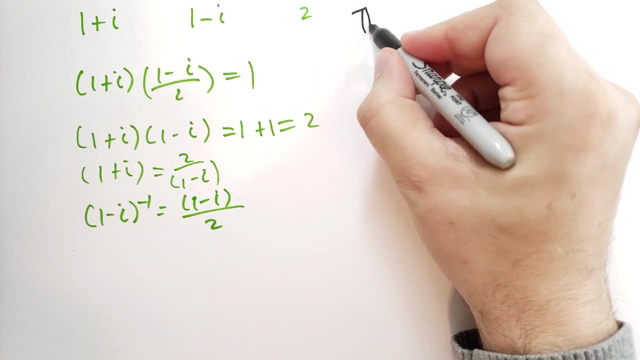 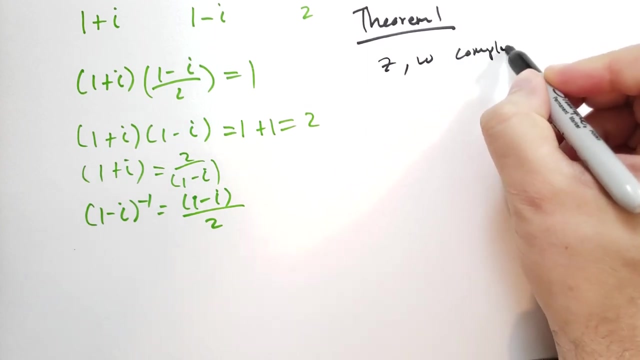 Okay, That's another way to do it. Many, many different ways to think about this. Okay, Theorem 1.. Theorem 1 says: let z and w be complex, Then z, w multiplied together first, and then taking the conjugate of it, is the same as multiplying the conjugates together. 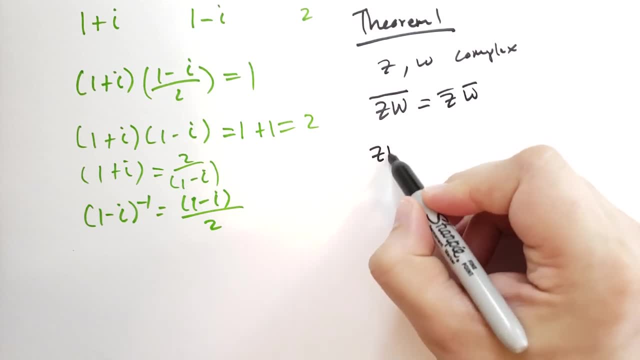 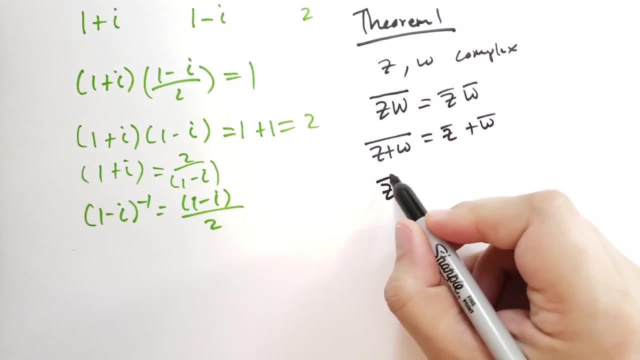 Okay. Also, if you add z and w together first and take the conjugate, that's the same as the sum of the conjugates. Okay. Also, if you take the double conjugate, you're going to get the original number back. 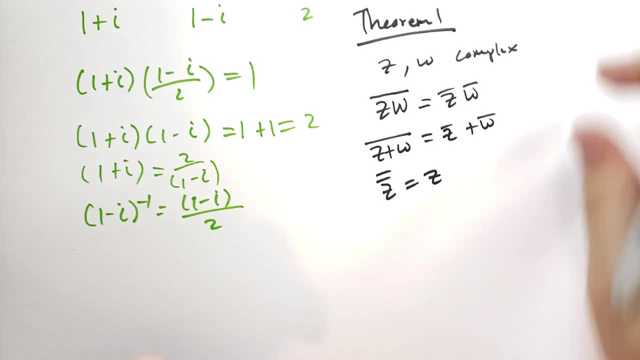 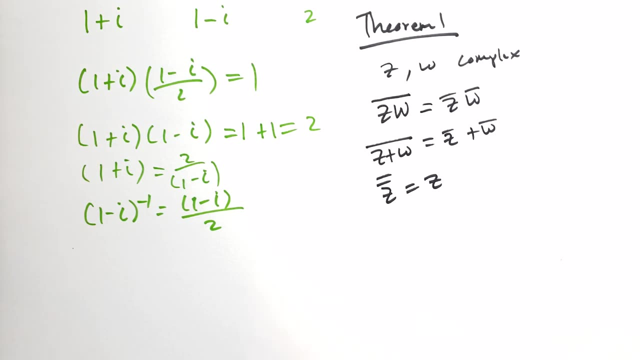 We're not going to prove this. It's rather trivial to prove, but this is something I think he leaves as an exercise. So go ahead and do that for fun, Figure that out on your own, Convince yourself of that Last little thing that we're going to talk. 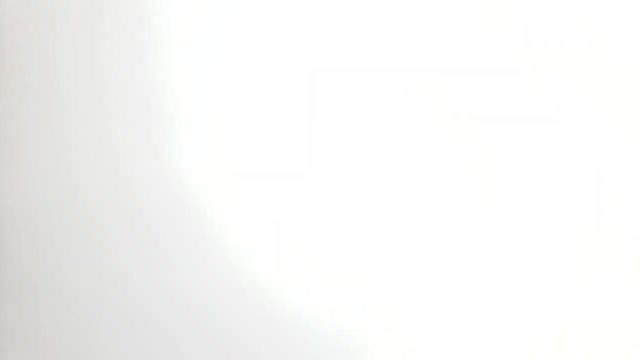 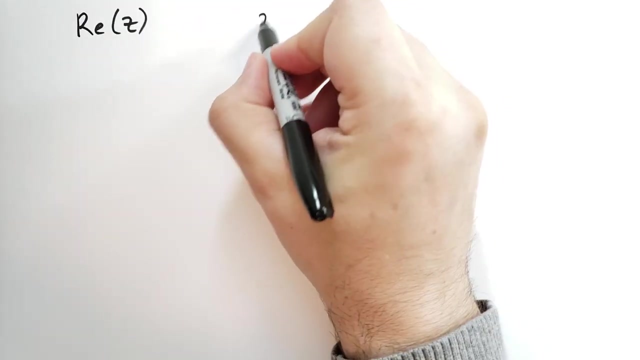 Two little things, Three little things, Okay. One: we sometimes use this, We say real of z, Okay, And that is going to give. if z is equal to a plus bi, then this is going to give you a, a real number. 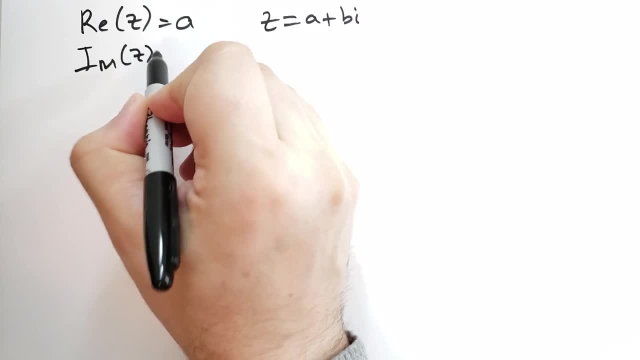 Okay, And we use m for imaginary of z and that's going to give you b, a real number. So the real and imaginary parts are in fact real numbers. Okay, If we have z is equal to a plus bi, then we take z and add that to the conjugate. 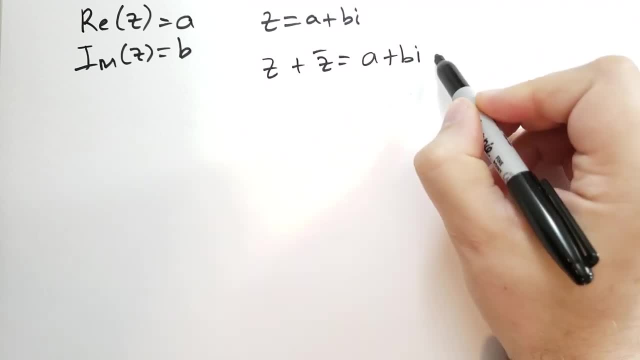 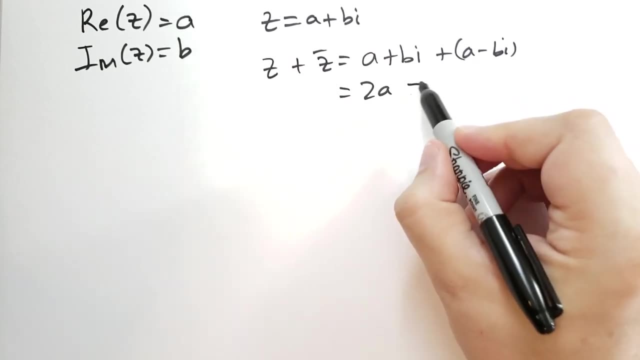 What's that going to give you? That's going to give you a plus bi, plus a minus bi, and that's going to be two a's. These two terms are going to cancel, So that's going to be twice the real part of z. 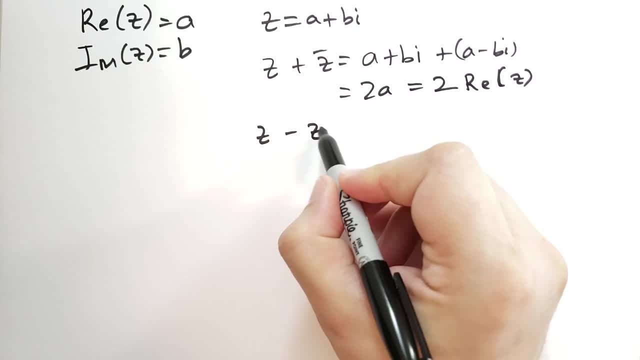 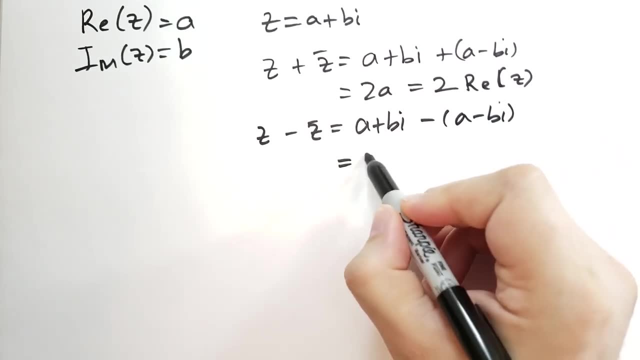 Okay, And if we take and subtract The complex conjugate, we're going to get a plus bi minus a minus bi. So we get a plus bi minus a. distribute the minus sign plus bi, So this is going to give you two bi, which is going to give you twice the imaginary of z times i. 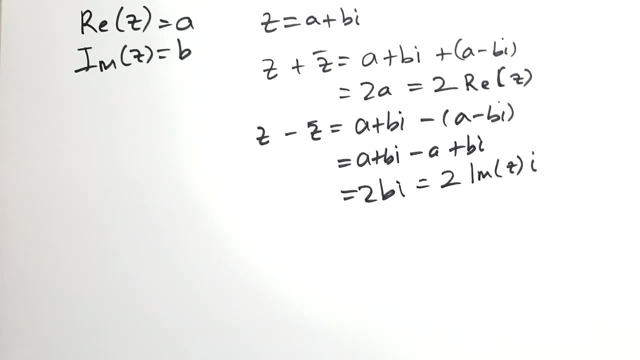 Okay, He has it in the book. I think he did it wrong in the book because he says z minus the conjugate of z is equal to two, y is equal to two times the imaginary of z. This is wrong because he's forgotten the factor of i. 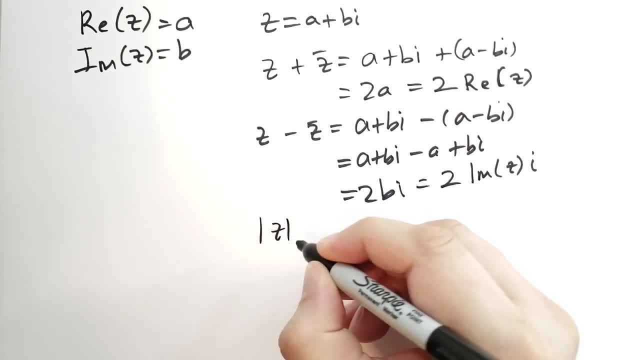 Okay, We also have the absolute value of z. Absolute value with real numbers is just, you know, flipping the negatives to positives and keeping the positives positive. You can think of the absolute value as the distance from the origin on the number line to that point in the real line. 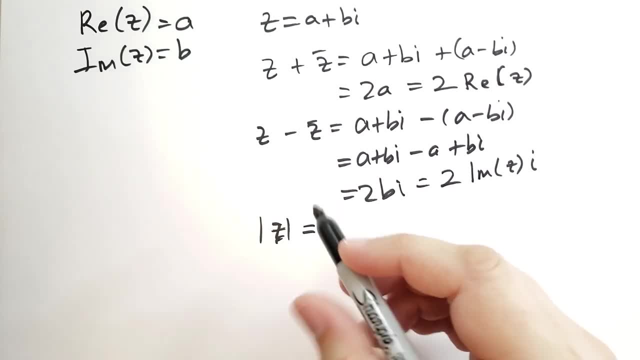 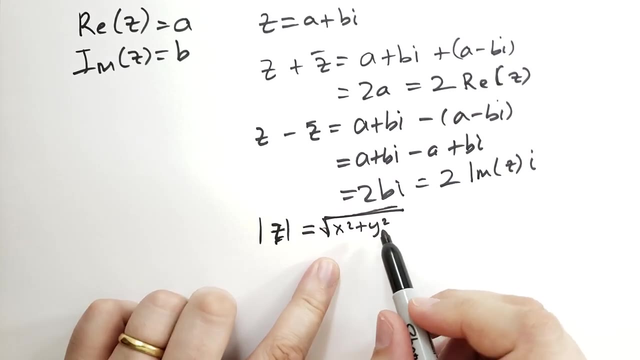 So the real number on the line, In the case of complex numbers, this is going to be the square root of the square Right. So if we take square root of the square Right, In this case the square is the x squared plus y squared is the square of the distance from the origin to the point. 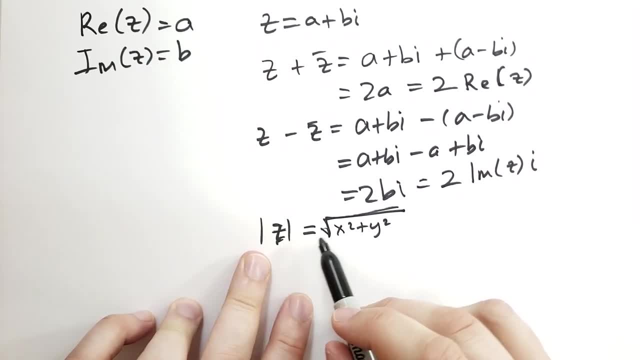 And so the absolute value of a real number is in fact the distance from the origin. If I can spell distance from the origin, Okay, We can calculate the inverse rather easily. It's just going to be the conjugate of z divided by the absolute value of z squared. 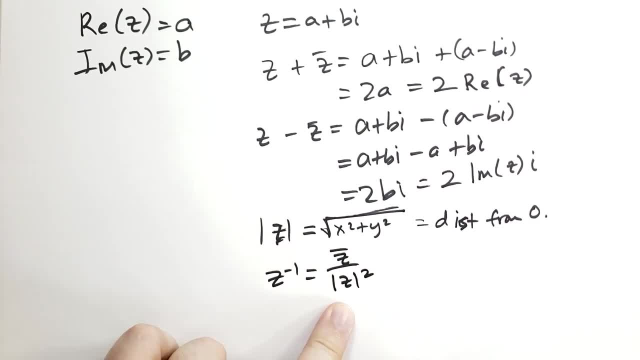 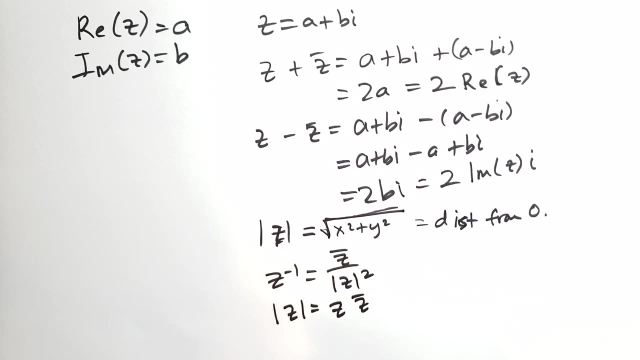 Okay. So if you know how far the point is from the origin, you can just square that. You can take the complex conjugate and get the inverse of that. Another way to calculate this is: we note that if we take the number times the complex conjugate, that's going to give us the square of the distance. 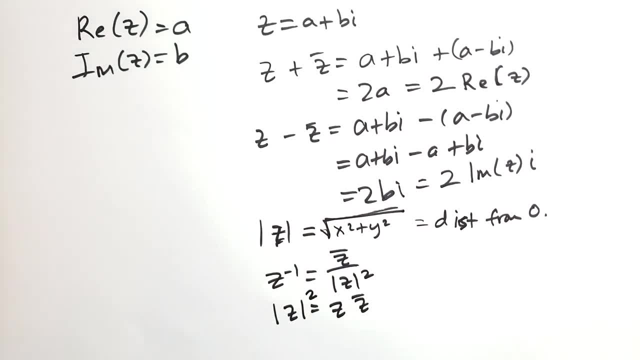 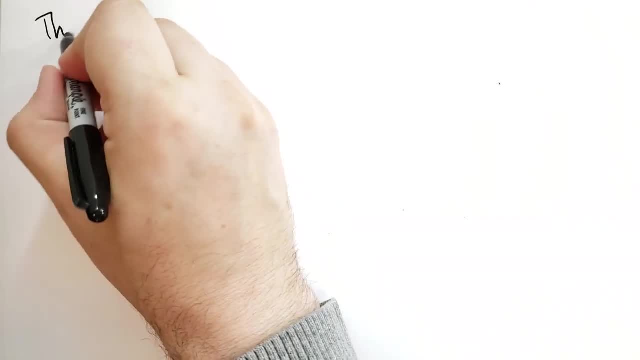 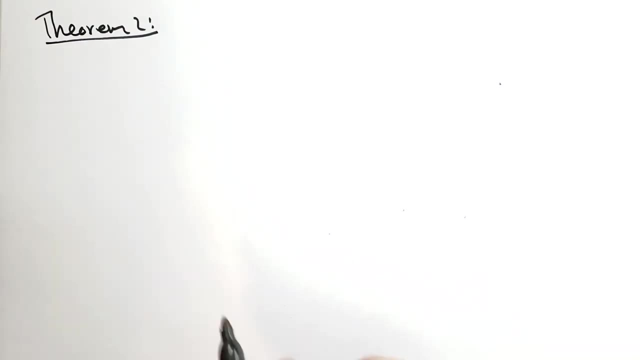 So this is the absolute value squared of z times the complex conjugate. Okay, Last proof, Last theorem. This is rather easy to prove. This is called 2. Theorem 2 in this section. He says the absolute value of complex numbers satisfies the following properties: 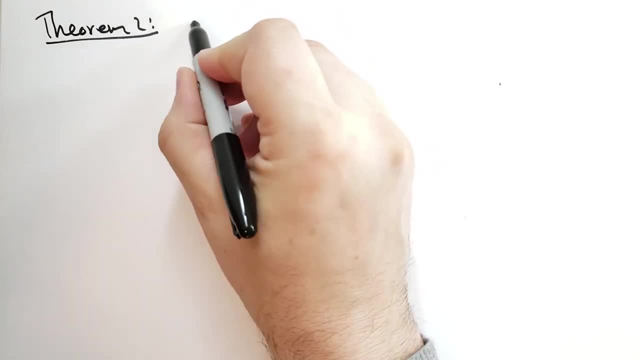 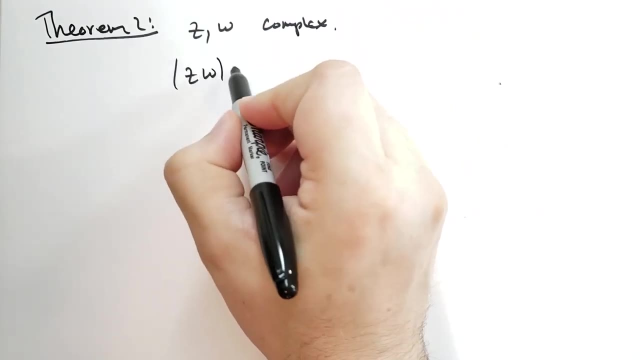 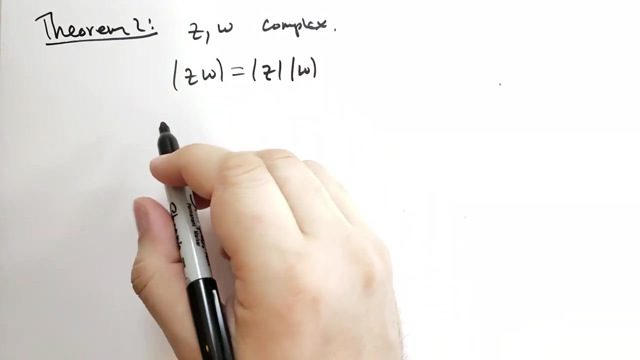 If z and w are complex numbers- so z and w are complex- then the absolute value of z times w is equal to the absolute value of z times the absolute value of w. This is rather an interesting result. actually, If we sum z and w, take the absolute value of z.